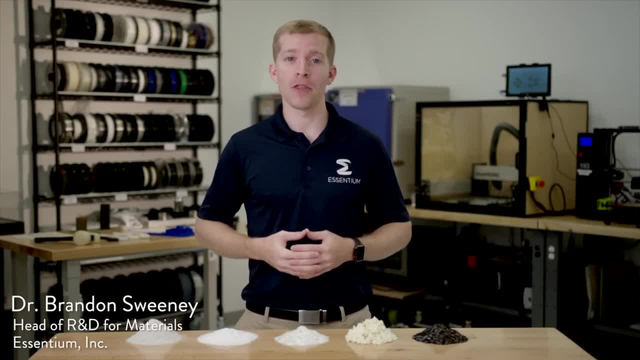 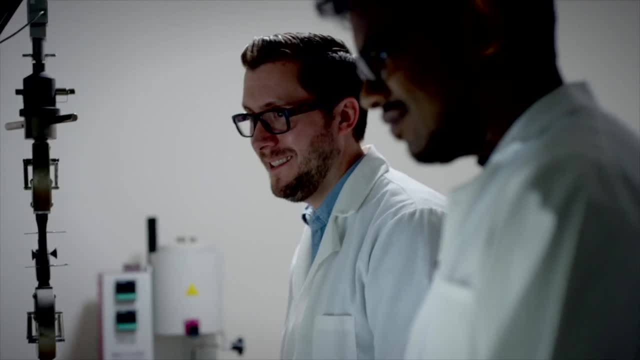 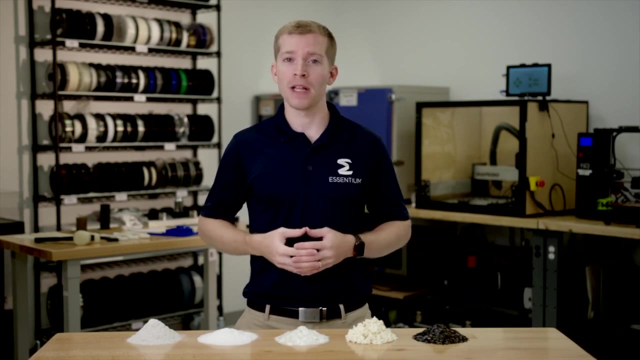 Hi, I'm Brandon Sweeney with Ascentium, and today we're going to learn about thermoplastic composites. A thermoplastic composite is a mixture of a thermoplastic polymer matrix and a functional filler material. The benefit of a composite material is you're able to combine material. 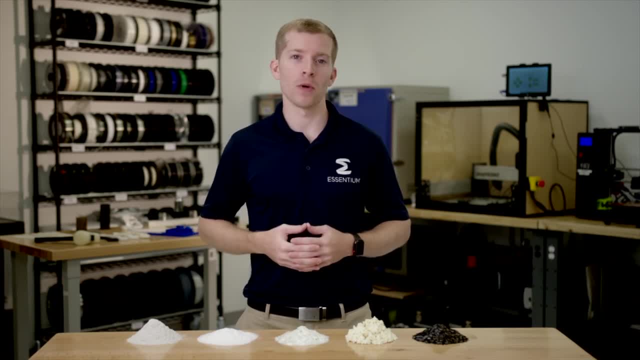 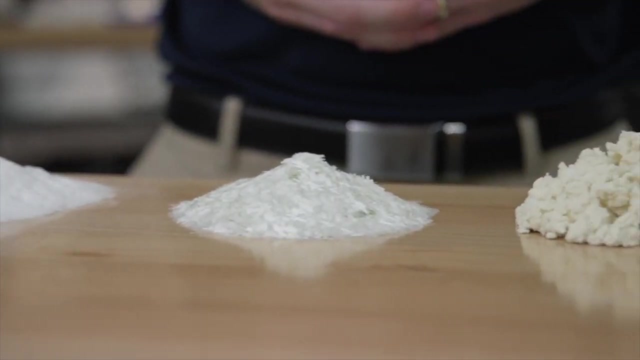 classes which yield unique properties not achievable with either material individually. Generally, composites tend to be high performance materials with higher strength and stiffness at a lower density, but they can also solve problems like wear, temperature creep and impact resistance. Common fillers include minerals like talc, hollow glass, spheres and chopped fibers such as glass. 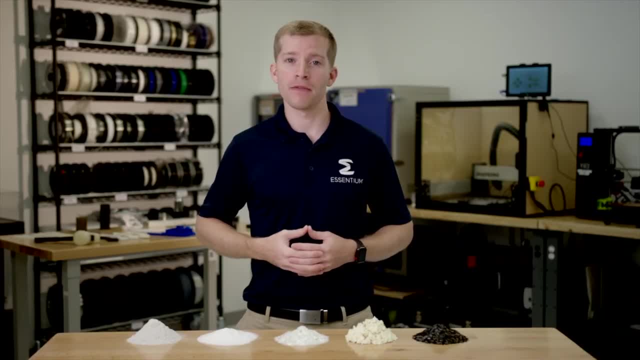 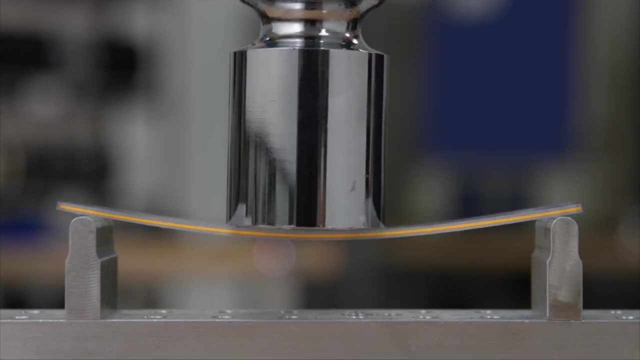 aramid and carbon Fiber fillers are especially effective at increasing the potential of thermoplastic composites, the strength and stiffness of polymers. Here you can see the difference in stiffness between unfilled PET, glass fiber PET and carbon fiber PET. This stiffening effect is achieved by 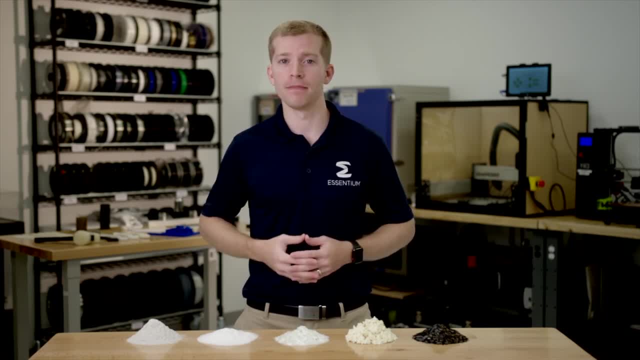 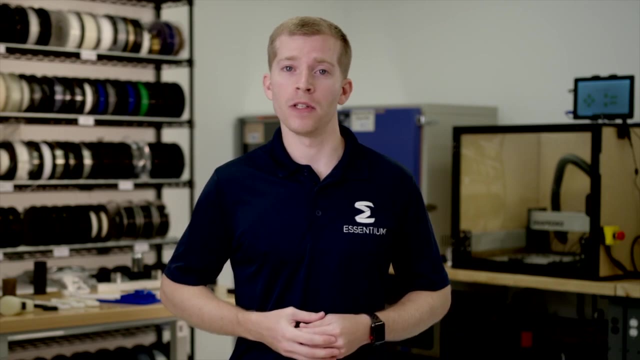 transferring stress from the polymer matrix to the fiber. The fiber reinforcement has tensile properties several orders of magnitude greater than the polymer matrix, so the properties of the resulting composite are somewhere in between the matrix and the fiber. The best way to utilize fiber fillers is to have a continuous thread aligned in the direction of the mechanical load. 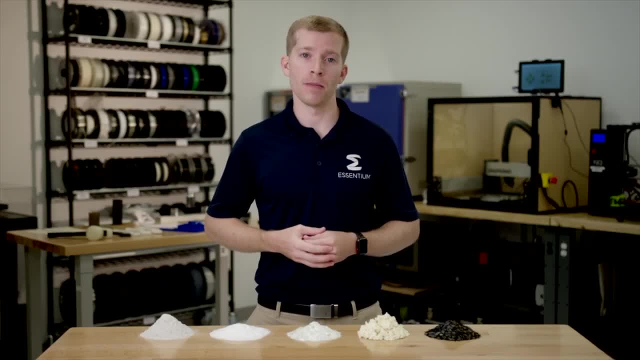 While some printers on the market can print continuous fiber parts, the cost and time it takes to print with this method is typically 10 times greater than a discontinuous fiber equivalent, making it impractical for everything but aerospace and exotic parts. Chopped fiber. 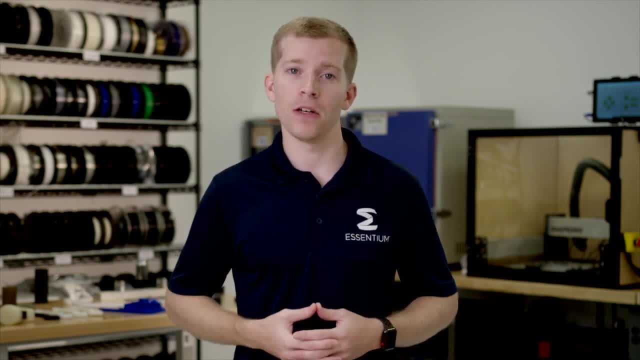 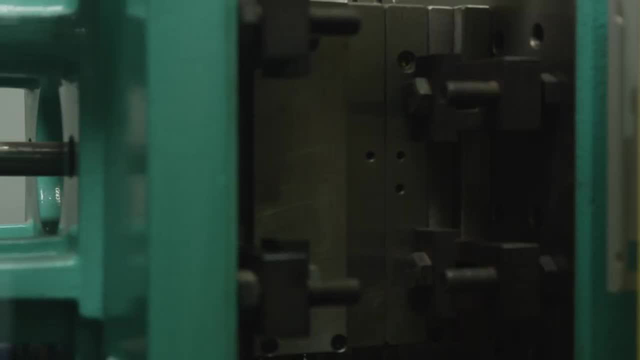 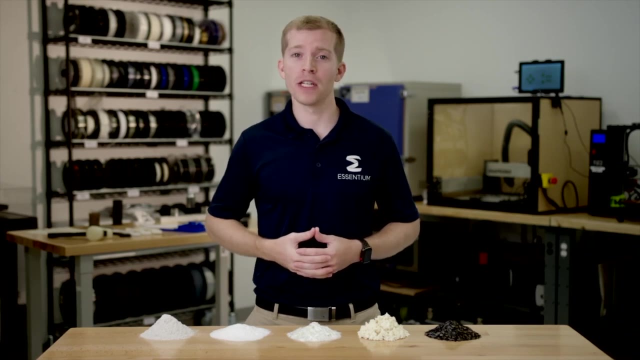 reinforced thermoplastics enable manufacturing at scale because the material costs are much lower and the production speed is much higher. by using continuous fiber fillers, These same benefits are realized for material extrusion 3D printing. Maximum tensile properties are achieved with high fiber volume fractions, high aspect ratio, fibers above the critical fiber. 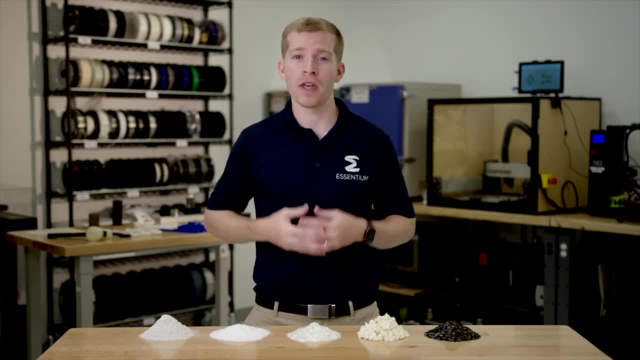 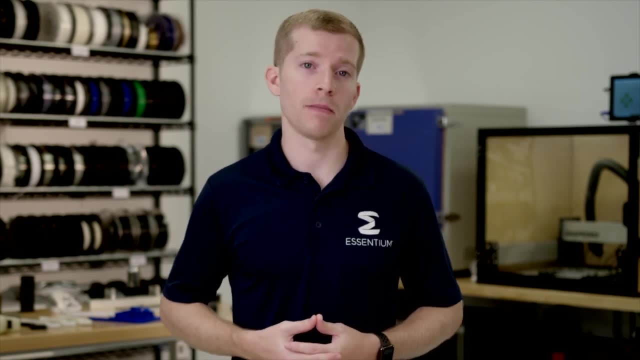 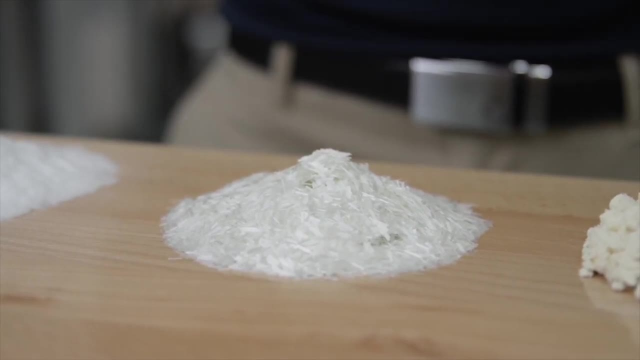 length and high modulus fibers and matrices with excellent interfacial surface chemistry for load transfer. Different kinds of fibers can impart a variety of properties to polymer composites. Glass fiber reinforced plastics have excellent price to performance ratio, along with good impact resistance, which makes them very 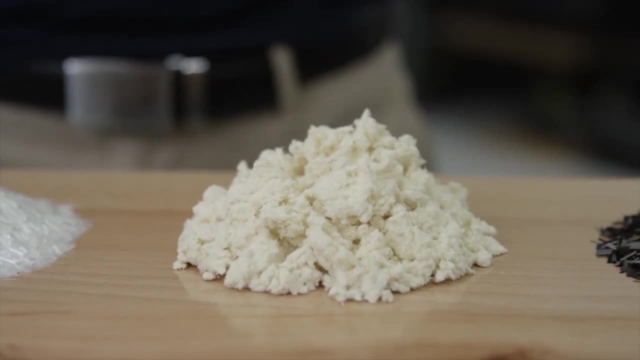 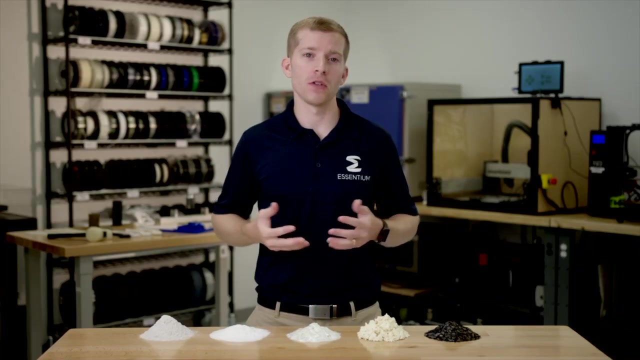 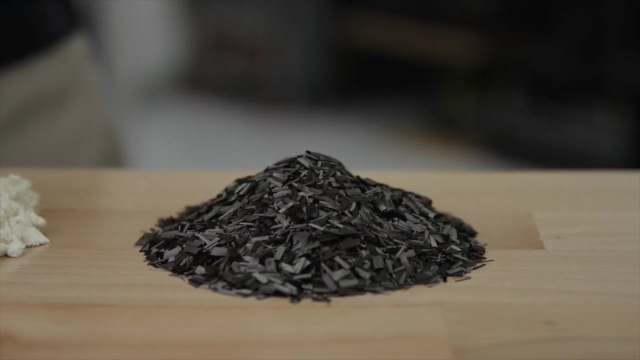 popular for automotive components. Aramid fiber reinforced thermoplastics are not as common, but tend to have outstanding wear and abrasion resistance, which makes them very useful for gears, bushings and bearings. Carbon fiber reinforced thermoplastics have the maximum performance for strength, stiffness and weight reduction, which makes them popular for aerospace. 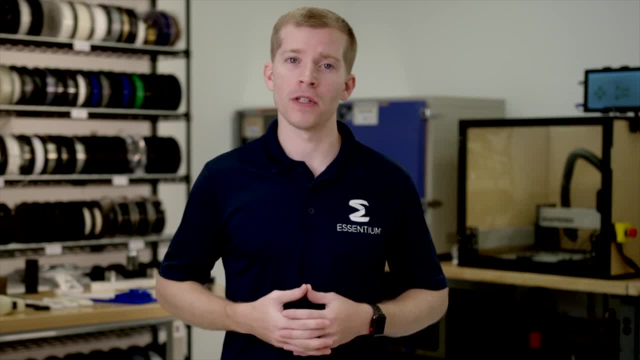 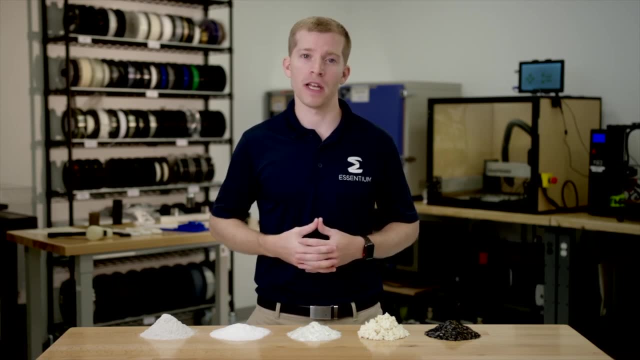 applications For 3D printing. carbon fiber filled materials are very popular because they are less abrasive than glass fibers and the carbon has a negative coefficient of thermal expansion and higher thermal conductivity than glass, which helps to suppress warping and shrinkage in printed parts. One thing to keep in. 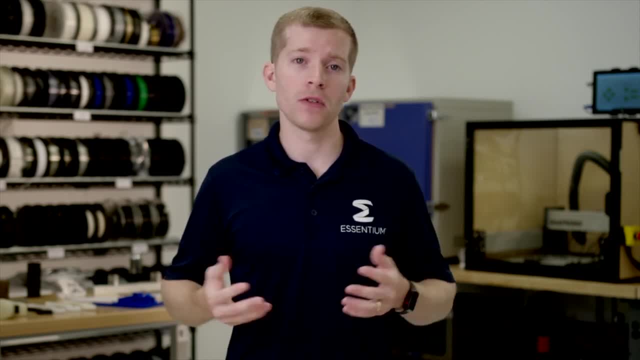 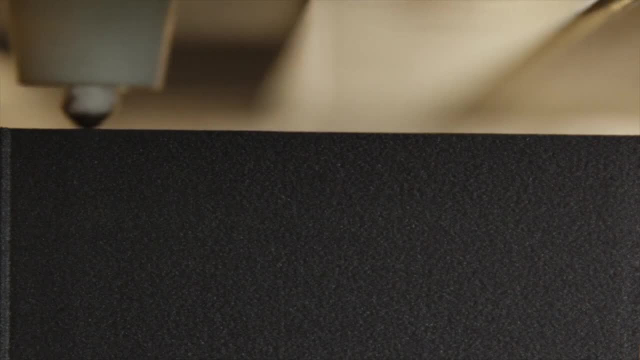 mind when printing with fiber reinforced materials is the flow-induced fiber orientation. As material is extruded from a nozzle, the fibers tend to align themselves in the direction of the flow and, as a consequence, you will see a long-term effect on the fiber reinforced materials. Carbon fiber reinforced material is 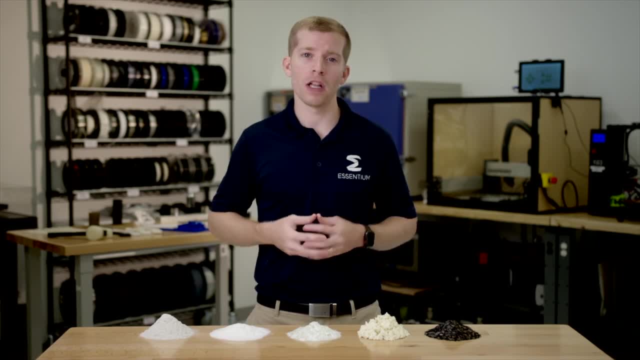 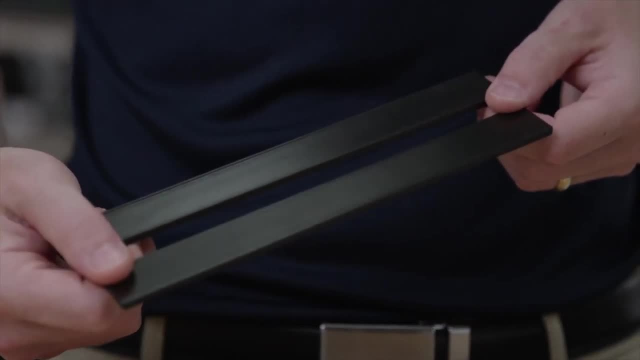 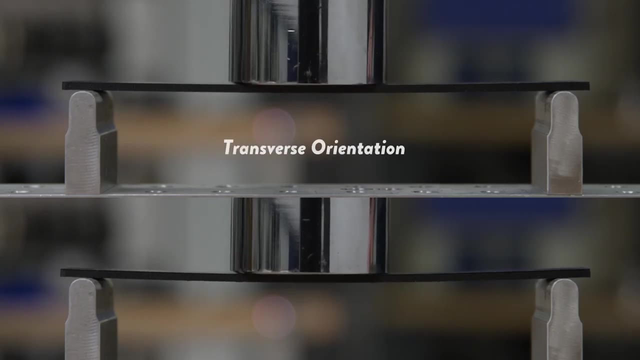 large difference in the strength and stiffness of parts where the polymer traces are oriented perpendicular and orthogonal to the print direction. Here we see a flex bar printed out of PET carbon fiber, with the traces aligned parallel and transverse to the loading direction. The bar with transverse. 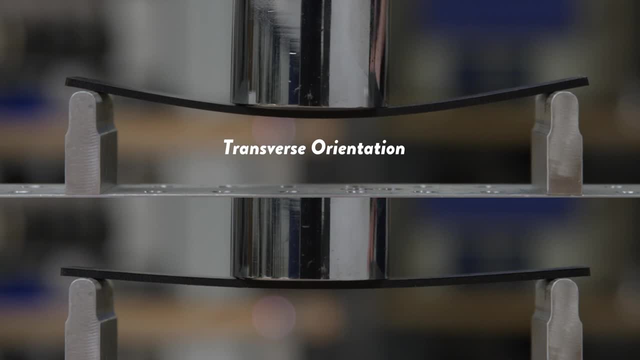 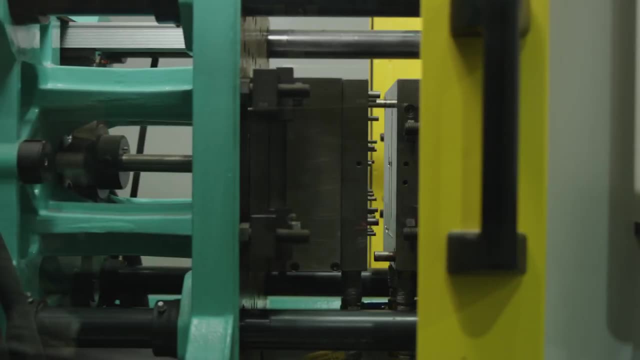 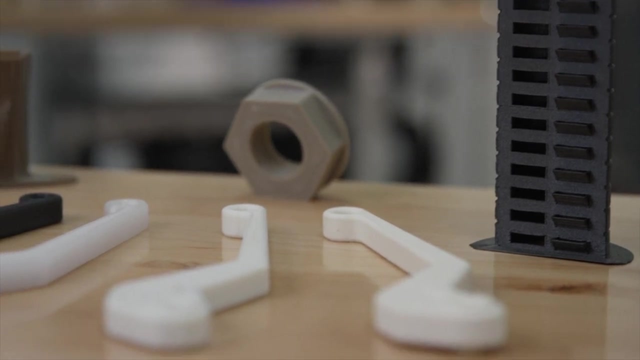 orientation has a much lower flexural modulus. This same effect is commonly observed for injection molded parts, and molders must take into account the machine direction and transverse direction and isotropy of fiber reinforced thermoplastics. At Ascentium we have a full line of fiber reinforced 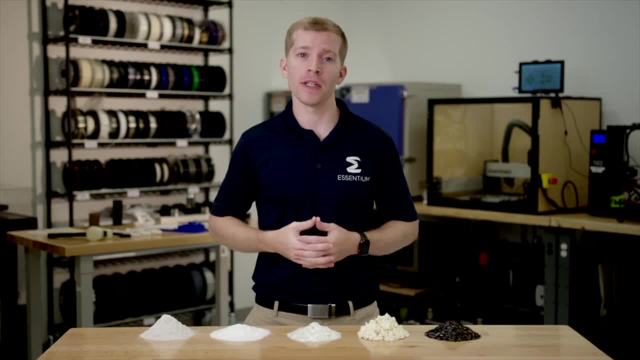 composites to meet your needs. One of our core capabilities is making multi-layer filament with an advanced co-extrusion process. With this technology, we've developed a 25% carbon fiber high temperature nylon composite filament by encasing it in a tough outer layer that helps to spool and feed the material. 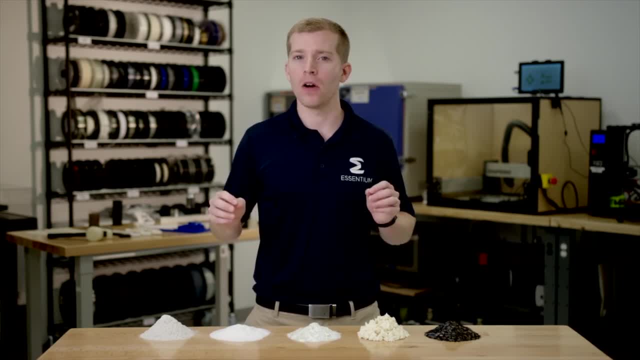 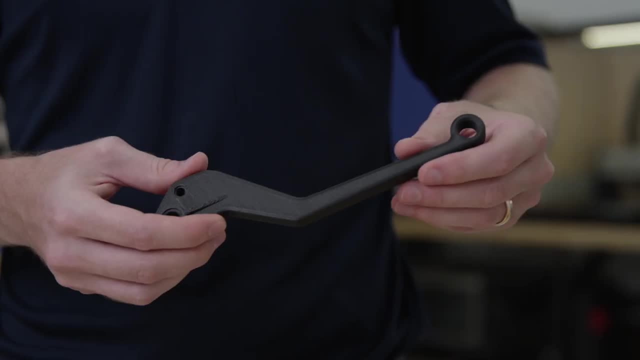 into the printer with a high-temperature nylon Without snapping the outer layer also reduces wear on your 3d printer feed section and nozzle, and it gives parts a silky matte finish. We love this material for its balance of stiffness and strength. It's perfect as a replacement. 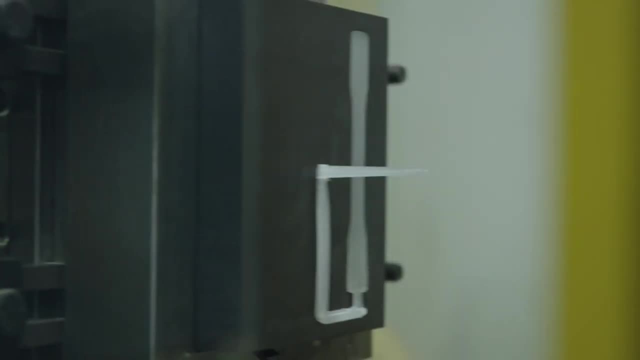 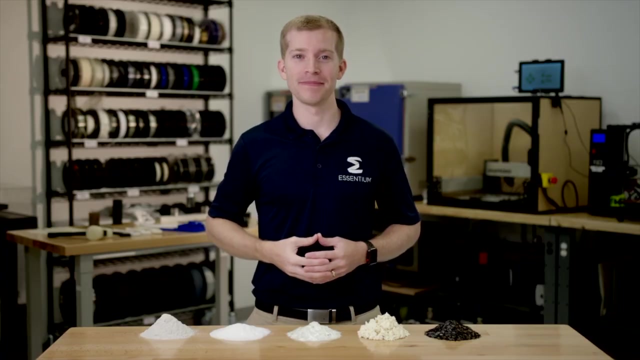 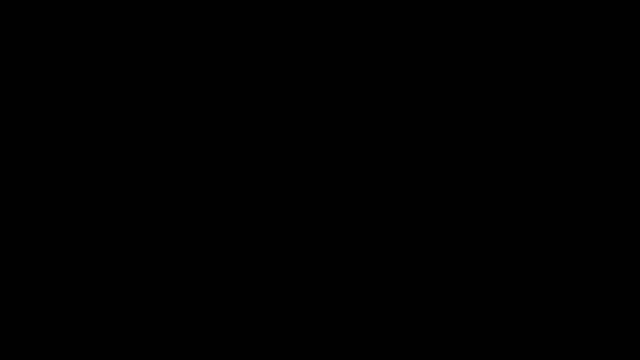 for aluminum parts and for making injection mold tooling. If you would like to learn more about our materials, please head to ascentium3dcom. slash materials- wwwascentium3dcom.